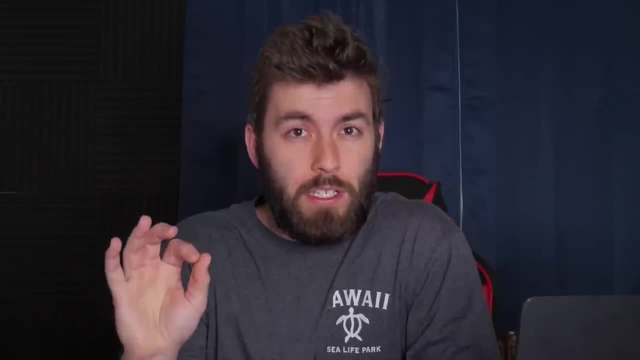 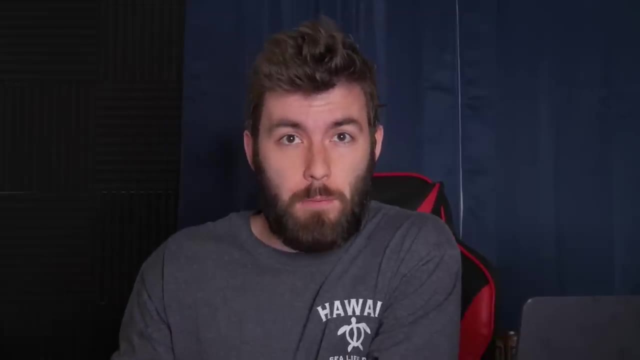 And then the physics major acts in a very similar way, but with one key difference being the reaction time. You see, the physics student is going to want to take some time to establish what assumptions they're making, but not for the sake of careful problem solving. 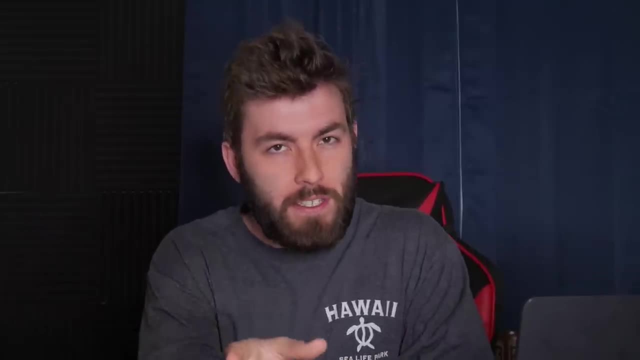 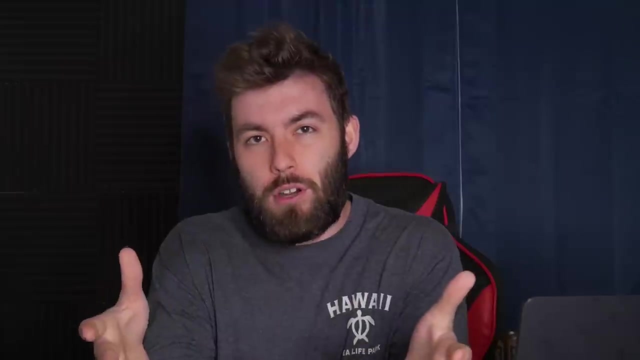 This is actually yet another defense mechanism. This way, the physics student can say something like: well, if those assumptions were valid, then I would have been right. But then, lastly, with the math major, they will say absolutely nothing and pretend not to know. 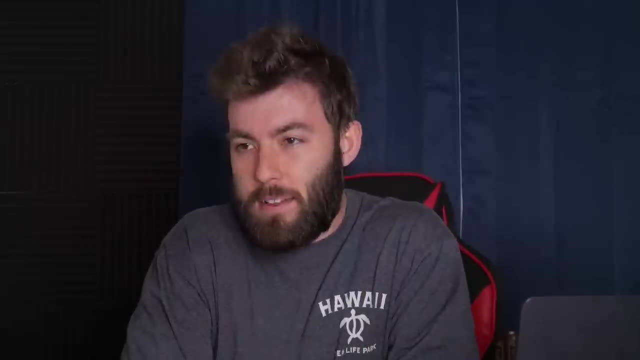 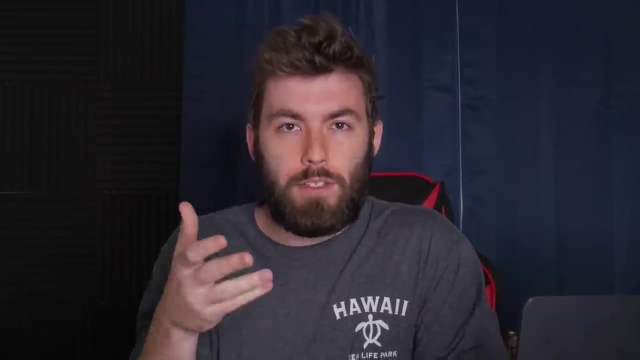 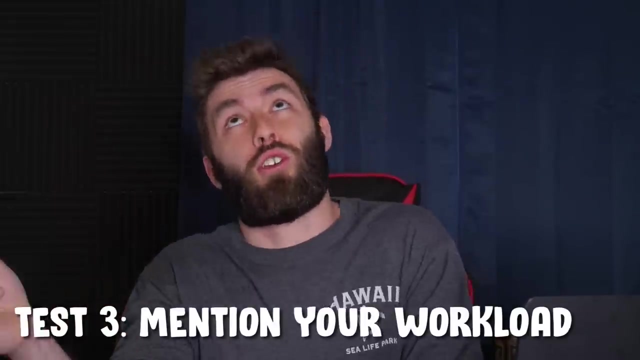 until they have 100% proved it for themselves. The math student is a very docile and passive breed until agitated through overconfidence in one's own level of rigor. That's when they are the most dangerous. The final test is to mention at some point how much work you have to get done. 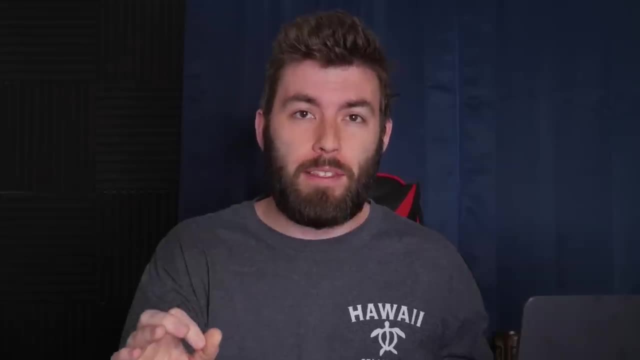 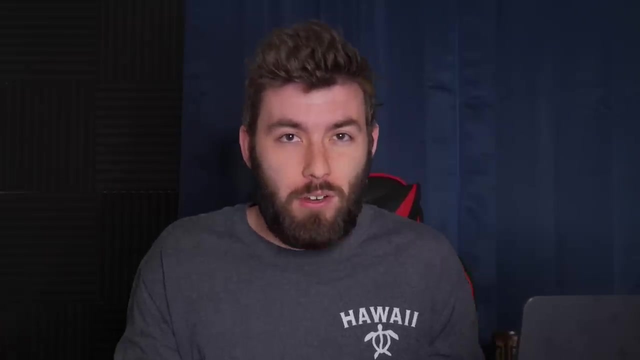 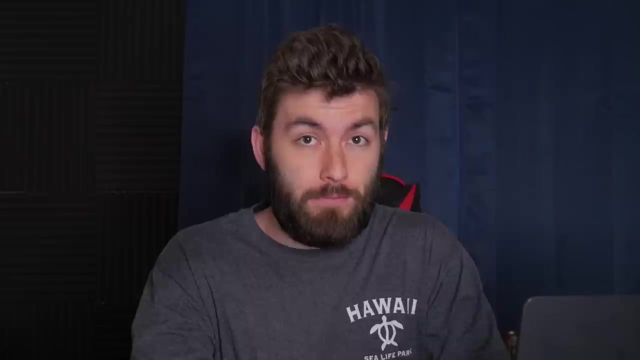 And, depending on your comfortability with confrontation, you should supplement this with mentioning also how difficult and challenging that work is. Now, both of these comments will trigger the engineering student and the physics major, but both comments to different degrees, so with the trained eye, a distinction can be made. 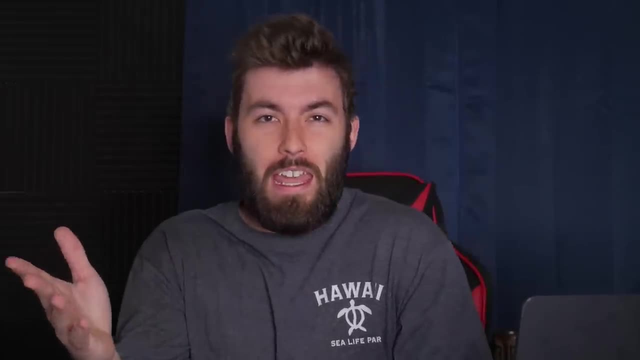 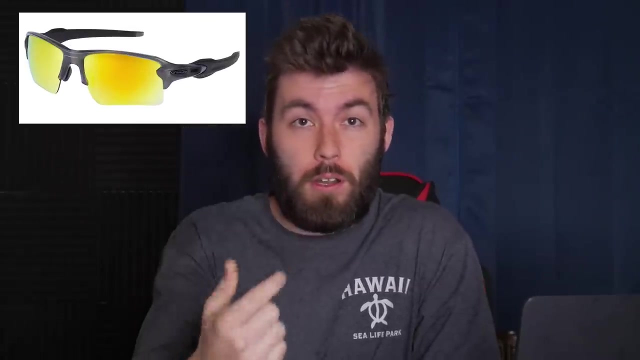 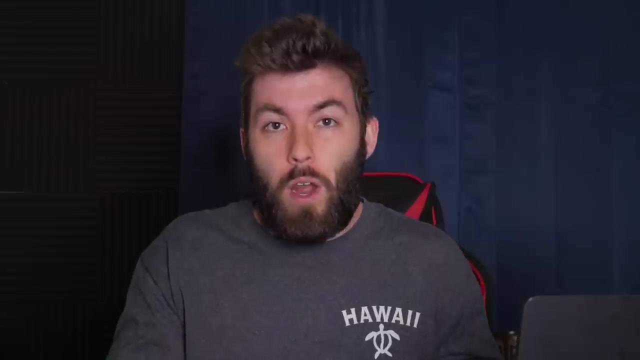 The engineering student will hear you mention how hard your work is and will feel challenged. Symptoms often include taking off their orange or yellow sunglasses with the bottom part of the frame missing, clenching of the jaw. You see, what they learn is often more tangible and easier to communicate why it's difficult than the physics major. 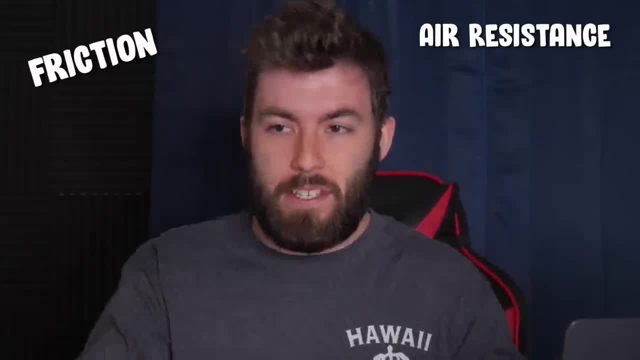 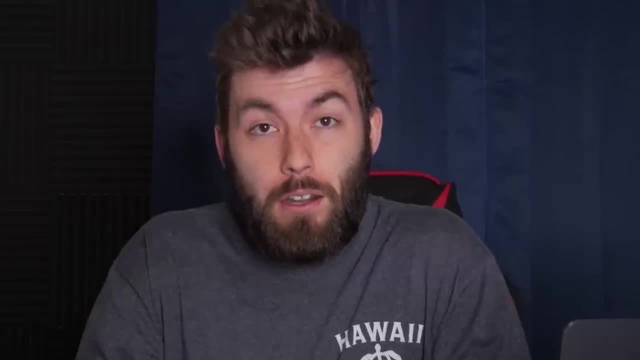 so you may hear something like: I had to account for friction and air resistance and efficiency and the strength of my material, So it'll be very easy to spot the pure rage building up in their eyes after that comment. The physics major, though, is a bit different. 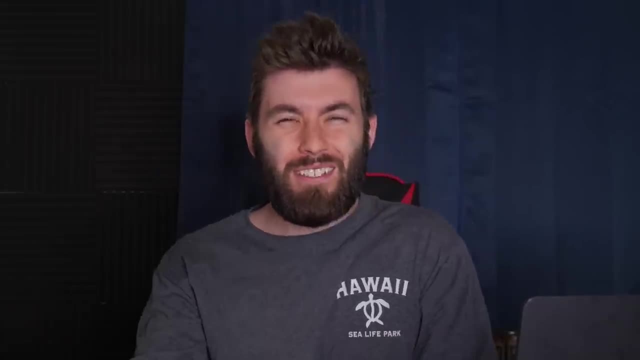 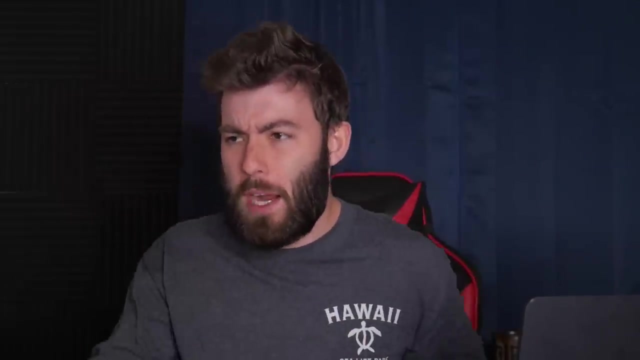 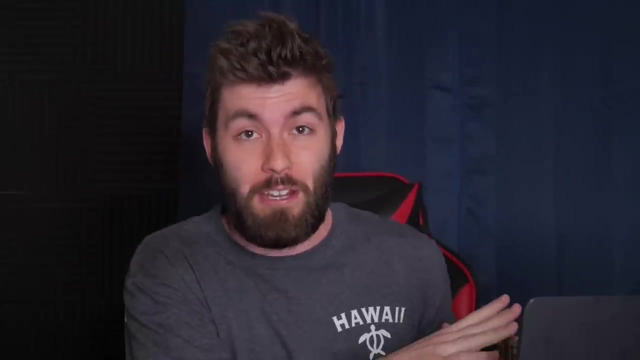 Things like abstract vector spaces mean nothing to most people, so giving the difficulty argument is just an uphill battle. So instead they will focus on the quantity, and then they'll immediately follow that by assuring you that everyone else in the class also had that much work and they weren't just over-complicating things. 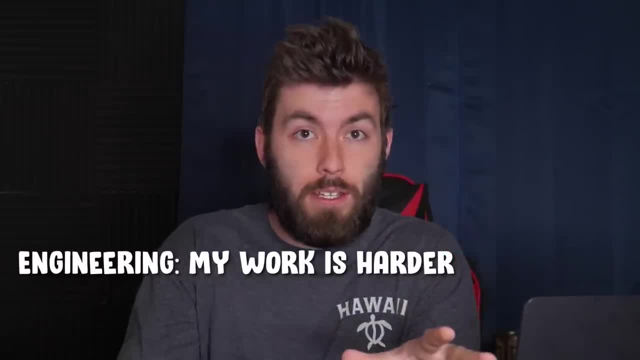 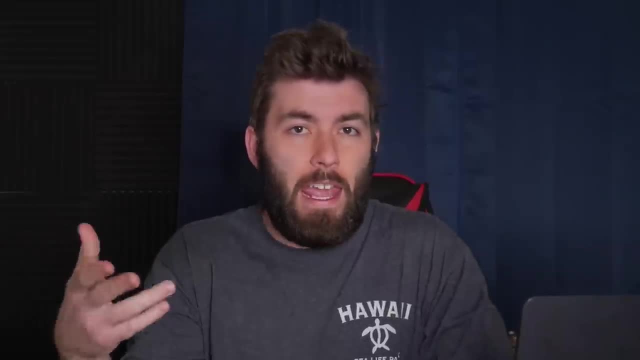 So the engineering student will be more triggered by how hard you said your work is, and the physics major by how much work you said it was. Now, if all else fails and you still don't know what kind of entity you're working with, they will pick up on it and they will tell you. they need to tell you, they need you to know.